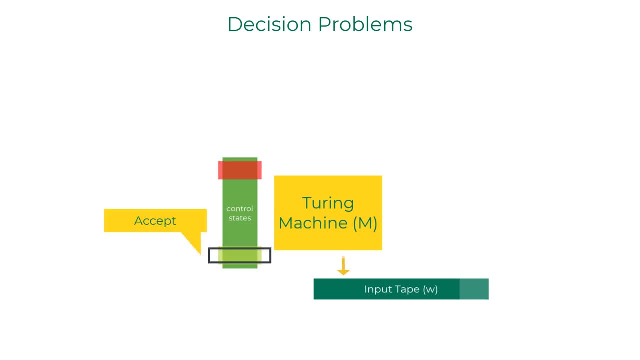 possible that the Turing machine can end up in an accept state on an input string. It is possible that the Turing machine can end up on a reject state on an input string. It is also possible that the Turing machine can end up in an infinite loop on an input string. The language of the Turing. 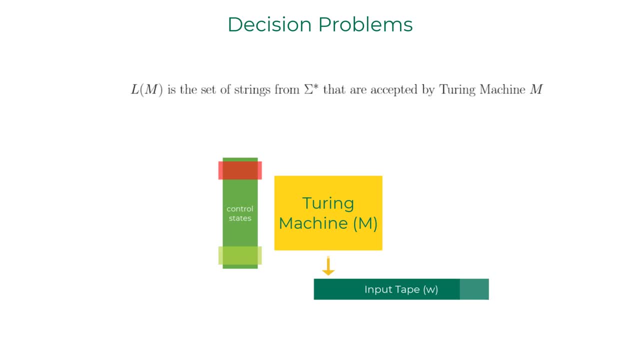 machine is the set of strings for which the Turing machine ends up in an accept state. If a Turing machine is a decider, then all the strings in Sigma star either end up in the accept or a reject state And the language of the Turing machine is called a decidable language. The class of undecidable languages is a. 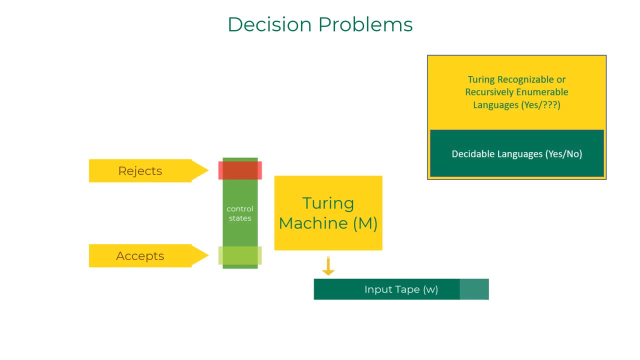 bit tricky to understand. Turns out that for few languages there exists a Turing machine that always ends up in an accept state for the strings that belong to the language либо푼, but may end up in reject state or loop forever on strings that are not in the language. So you 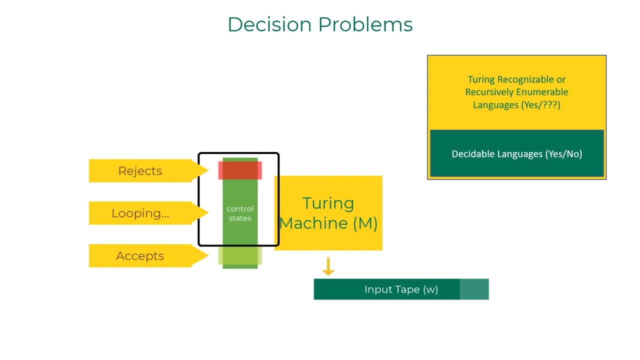 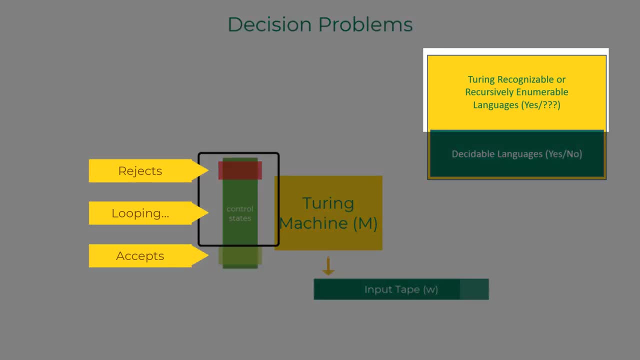 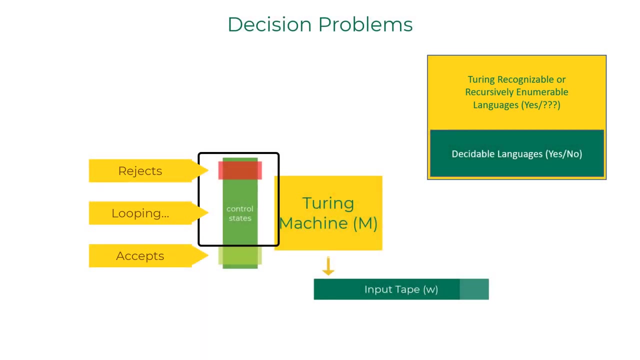 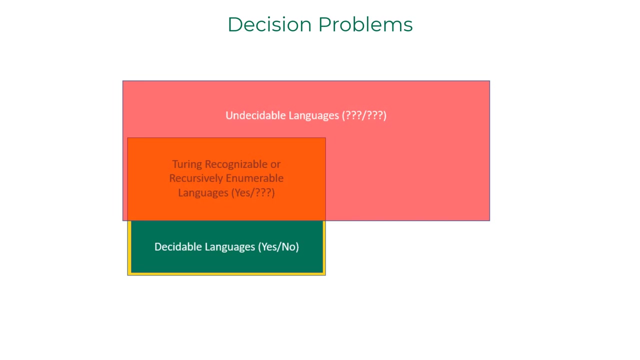 cannot get a definitive no for the strings that are not in the language. Such languages are called Turing recognizable or recursively enumerable languages, because at least you will get a yes for the strings that belong to the language. And then there are a few undecidable languages. 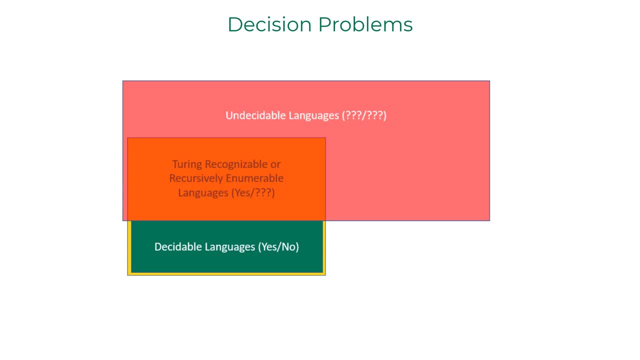 for which there exists no Turing machine that definitively ends up in accept state or a reject state. Hence Turing machines cannot even say yes for the input strings that belong to a certain language. These are the class of problems that are completely undecidable. 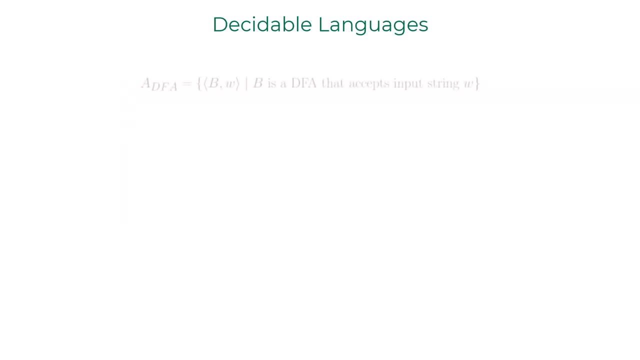 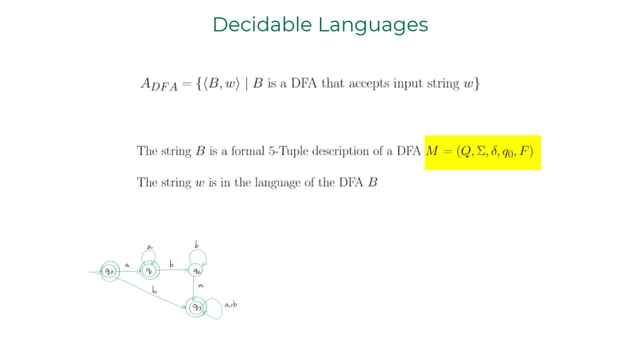 to construct and simulate a DFA. you would be able to construct and simulate a DFA If you were able. By looking at a 5-tuple using a pencil paper and an eraser. you can assume that a Turing machine can also construct and simulate it, given appropriate control instructions. 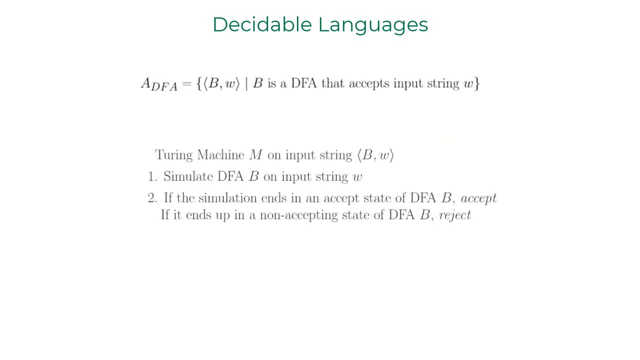 Here is the informal description of the Turing machine M that decides A DFA, First step. simulate B on input W. If the simulation ends up in the accept state of the simulated DFA, then end up in the accept state on the Turing machine. If it ends up in a non-accepting state in the simulated DFA, then end up in a reject. 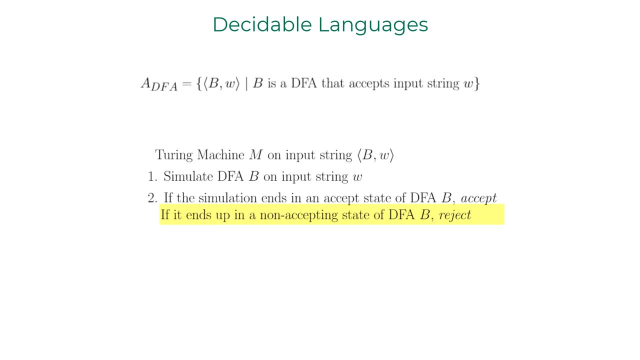 state on Turing machine For a string of a finite length. the finite automaton simulation ends in finite number of steps on the Turing machine, Hence A DFA. So you get a definitive yes or no answer for all the strings that are basically encodings. 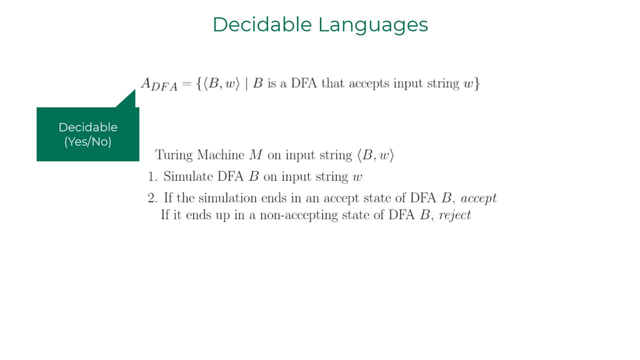 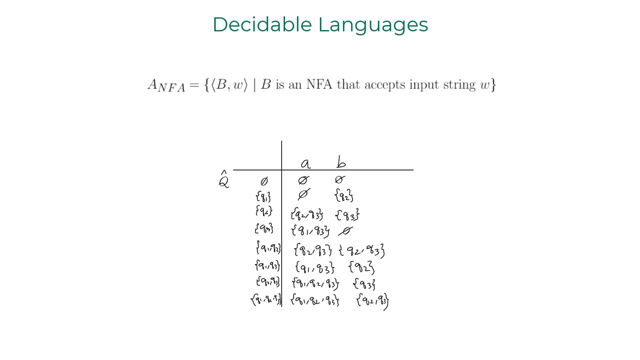 of a DFA and the word that they accept. Perfect. Now how about A NFA? Turns out. you can algorithmically convert an NFA to DFA using subset construction method, which you have learned earlier. Anything that can be algorithmically computed can be computed on a Turing machine, so you 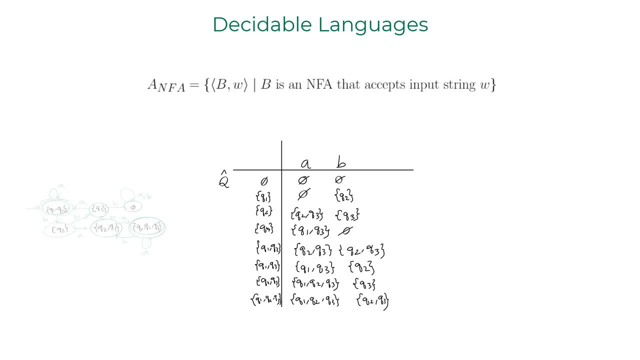 add an extra step of this NFA to DFA conversion and repeat the same procedure cited earlier. Now, how about A REGEX? Again, there exists an algorithmic procedure to convert a regular expression to an NFA which can be converted to DFA. 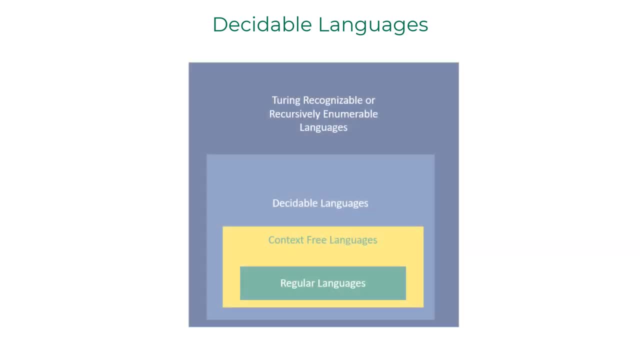 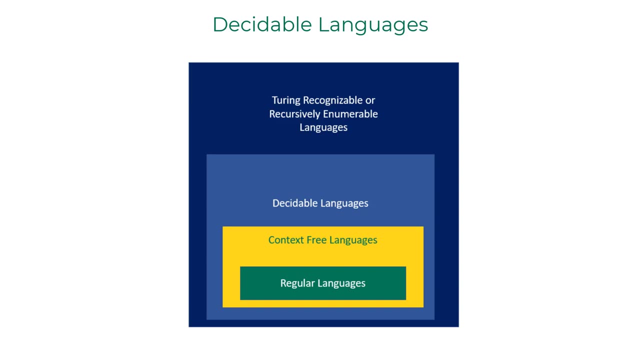 Hence A REGEX is decidable. Okay, Turns out, even context-free languages are decidable languages. Here is the relationship among class of languages that we have seen so far.